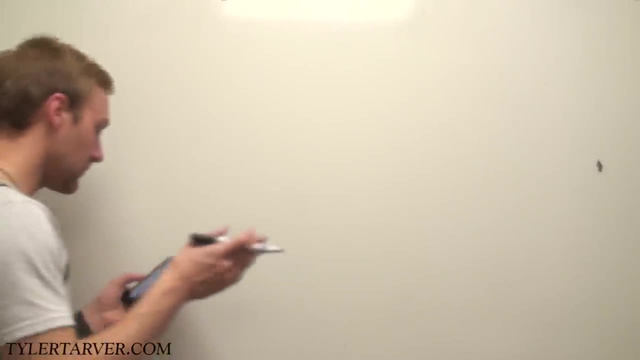 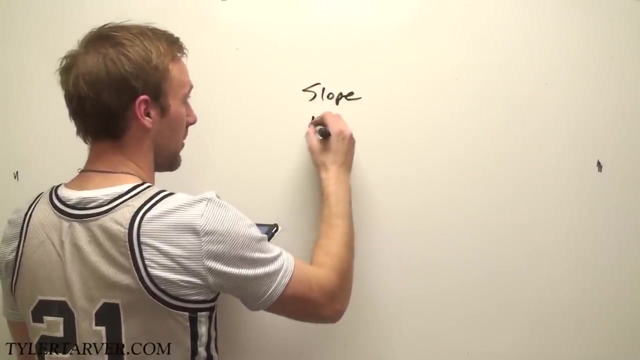 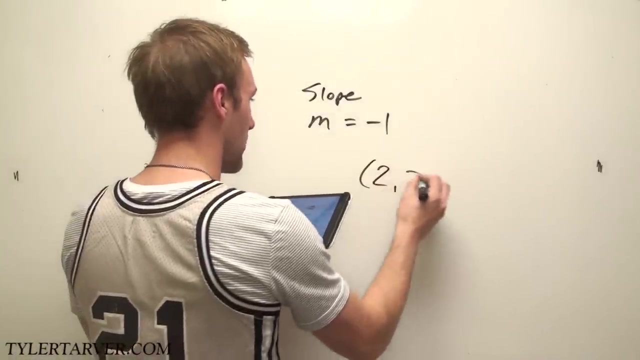 slope. okay, So I'm going to read the question and I'm going to work the problem. It says the problem is a line with a slope of negative 1, which slope is m equals negative 1, alright. And it says it passes through the points at 2, 3, and 5y, which that's an awful usage. 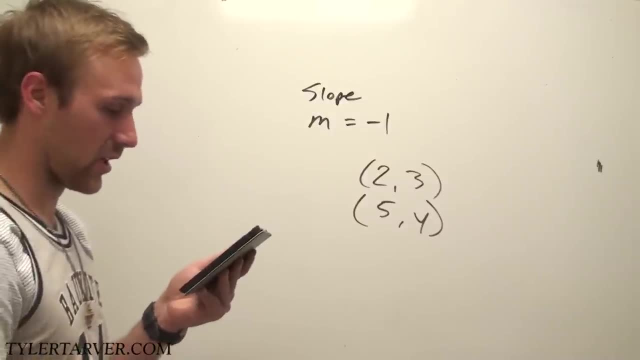 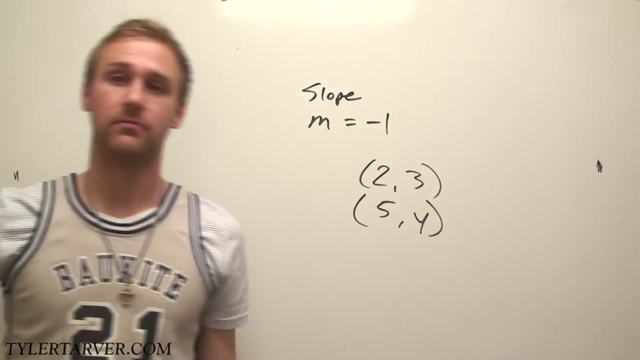 because you think, oh, y, and it's going to get confusing when you use slope-intercept formula etc. Find the value of y, Alright, well, let's work this problem. Okay, May the month. let's work the problem, okay. So we got this. Now there's a couple different ways to work it. 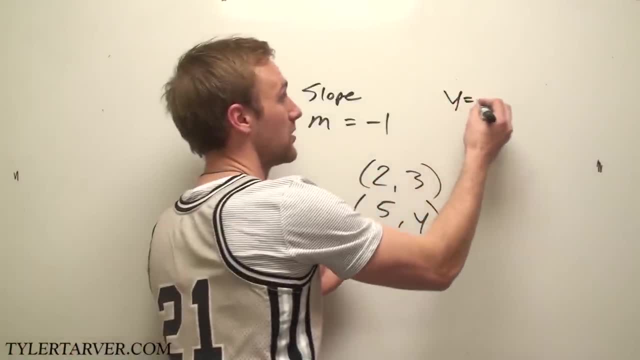 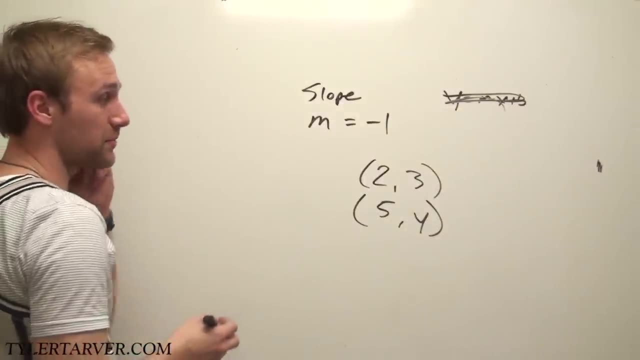 If you want to, there's a couple steps you can use in the slope-intercept formula, which is: y equals mx plus b. I don't think that's necessary. I think we can just use the slope formula. okay, So this is the slope. The slope formula is y2 minus y1 over x2 minus. 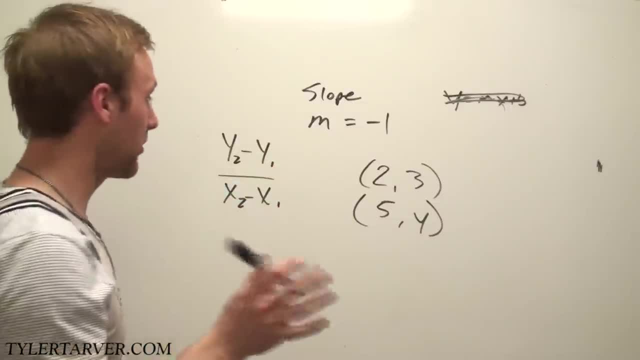 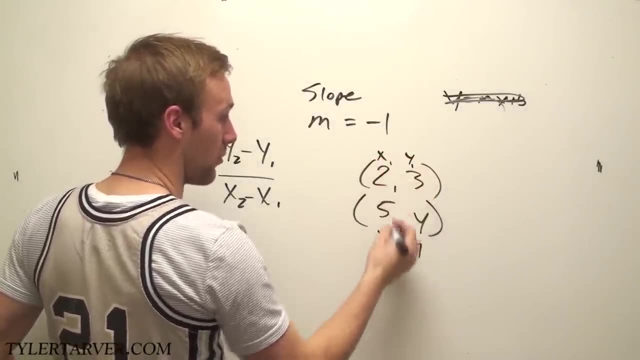 x1, correct, Okay. so what I always recommend to my students and everybody else: label this stuff. It's an x, this is a y, x and this is a y. This is your x1, because it's problem 1, x2, y2.. And I'm just going to separate those two because it's confusing, because there's. 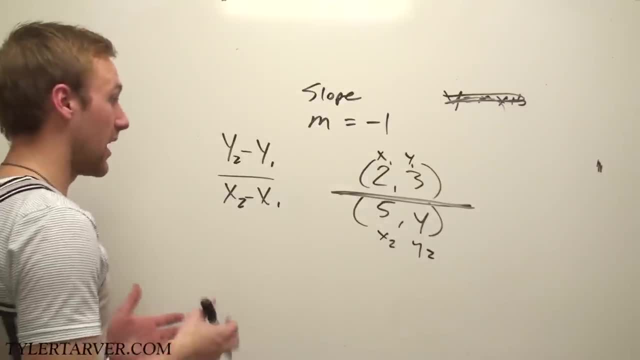 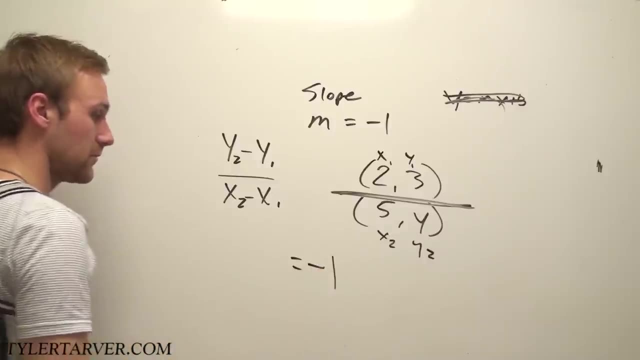 a y there, Whatever. Okay, so we plug our stuff in and we solve it. okay, We already know what it equals. We know our slope equals negative 1, okay, Cool. So now we just do the little thing I always say: We just plug in what you know. 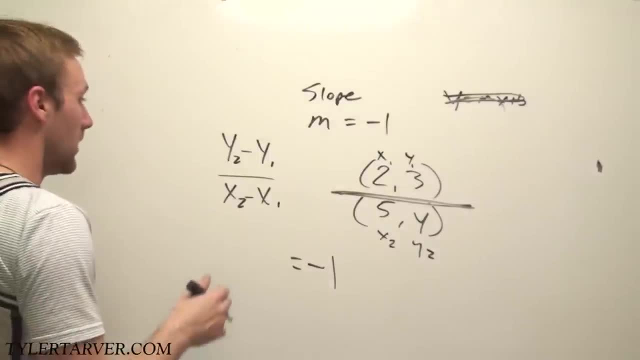 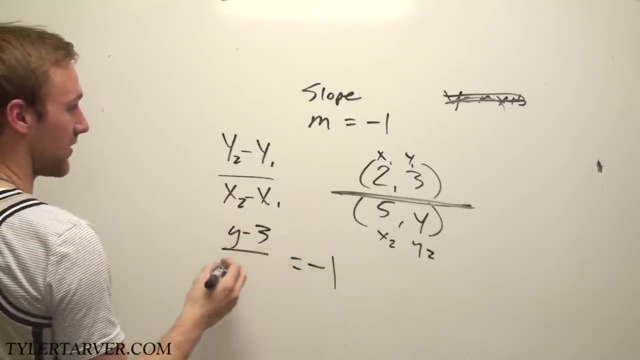 To find what you don't know. okay, Here we go. So let's plug in our stuff: y2 is our y minus our y1 is 3 over x2, which is 5 minus sine, x1 is 2.. So we simplify it. I can simplify. 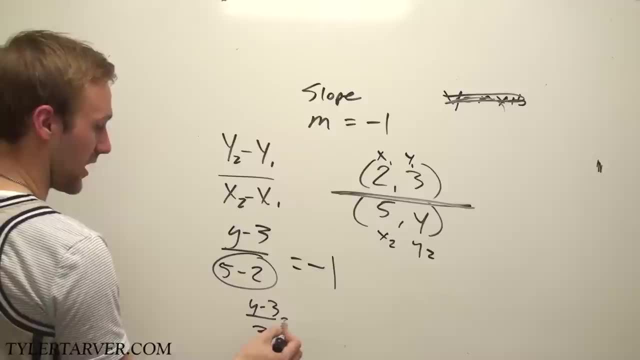 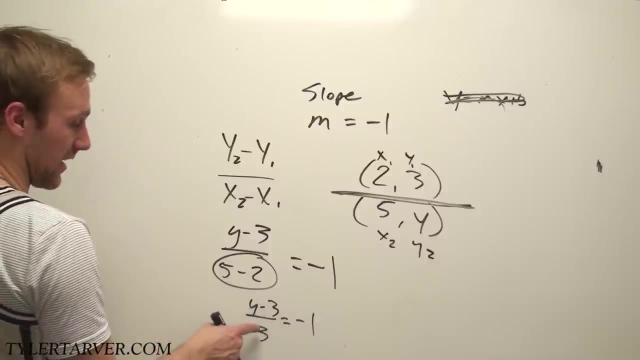 this, It'll be y minus 3.. 5 minus 2 is 3.. Now we've got to get rid of the stuff furthest away from y, which isn't the thing hanging out on the same floor as it It's going to. 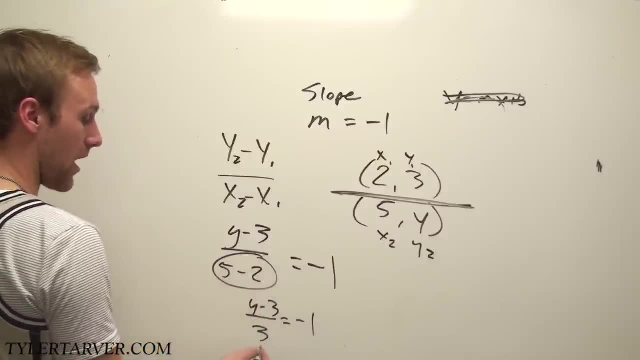 be that 3.. So how do you get rid of divided by 3? Multiple by 3.. So you're going to get to multiply both sides by 3.. That cancels out. We've got. y minus 3 equals negative 1. 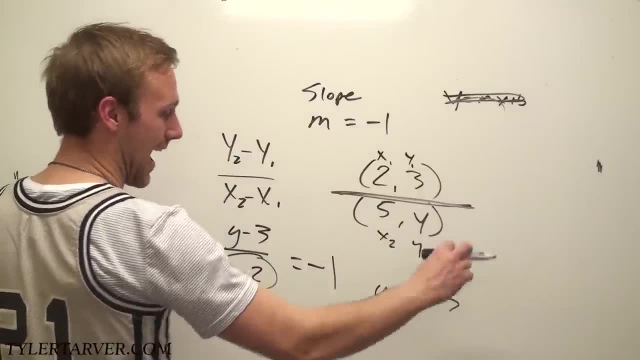 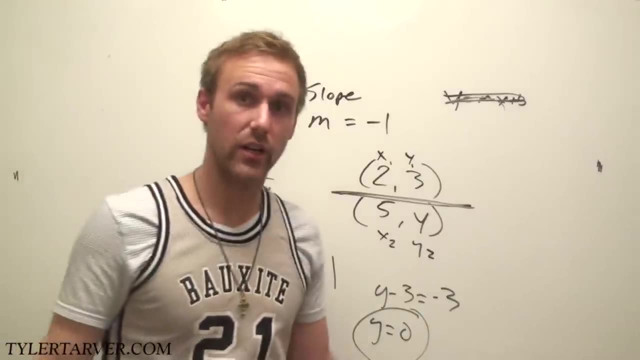 times 3 is negative 3.. What do I do to get rid of that 3?? Add it: Negative 3 plus 3 is 0. And you've got your answer. That's how you do it. Now do you want to check it? Sure. 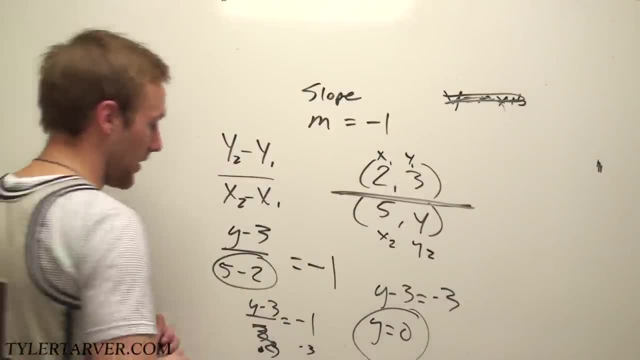 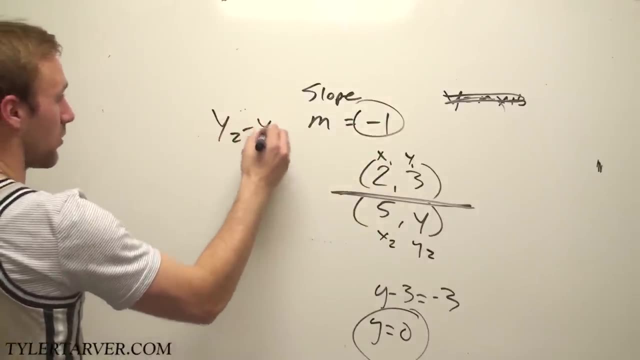 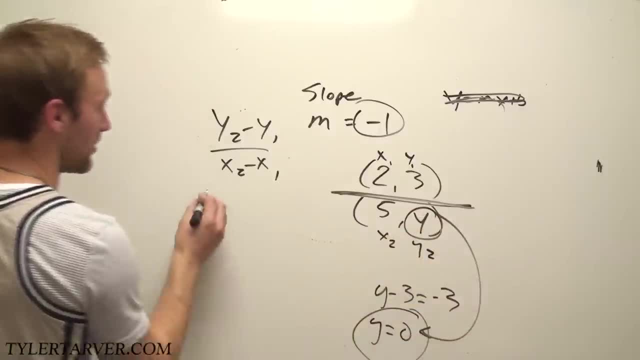 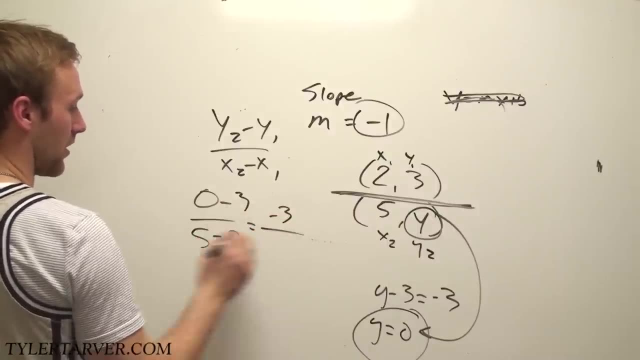 so it's going to be 0 minus 3 over 5 minus 2.. That will be negative. 3 over 5 minus 2 is 3, which simplifies Negative 1, that's what we want, That's what we've got, That's. 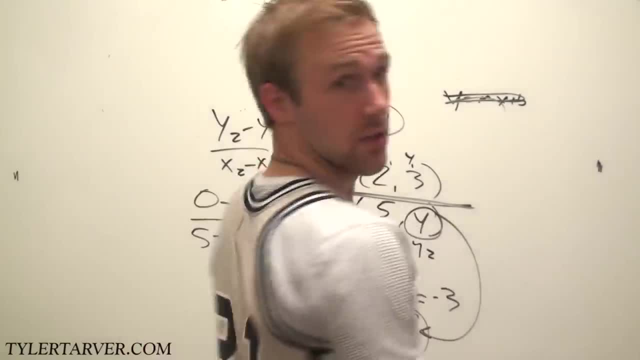 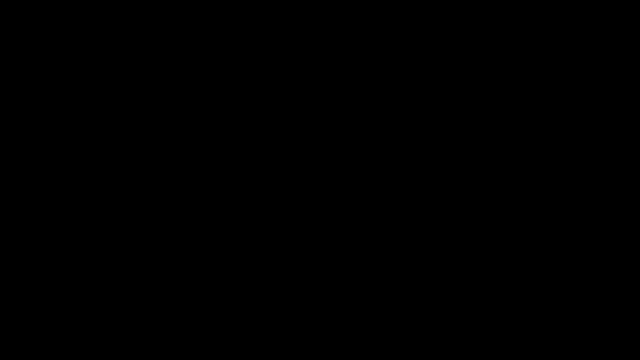 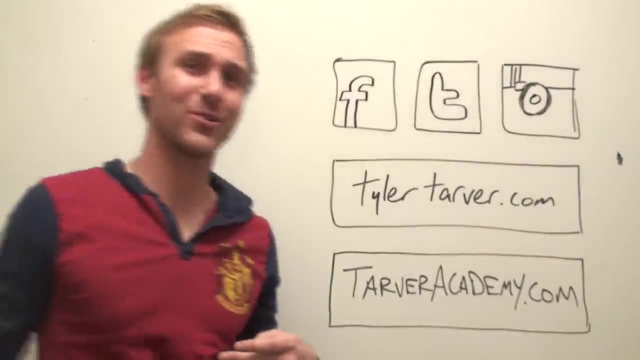 the finish of our problem. What up, Thank you for watching the video. I real, for real, appreciate that. you know I do. you know I do go okay, so if you could, real quick, I'm gonna run through, check me out on Facebook if you want to type. 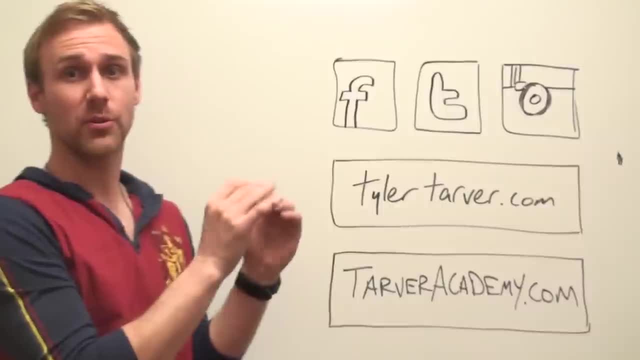 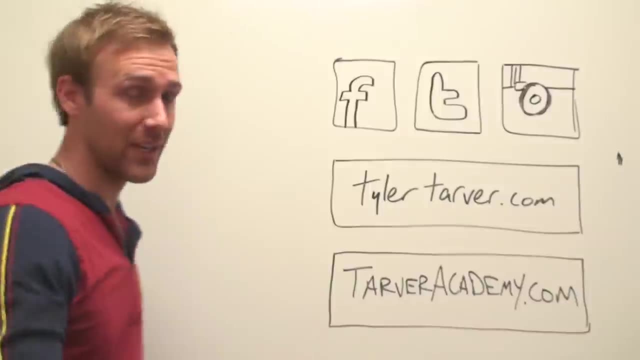 in Tyler Tarver to pop up? Tyler Tarver is okay, we're gonna just go facebookcom slash- Tyler's okay. or you can just do FB comm slash- Tyler's okay. yeah, Facebook jumped on. that got the FB calm. good job, Facebook. check me out on Twitter, Tyler. 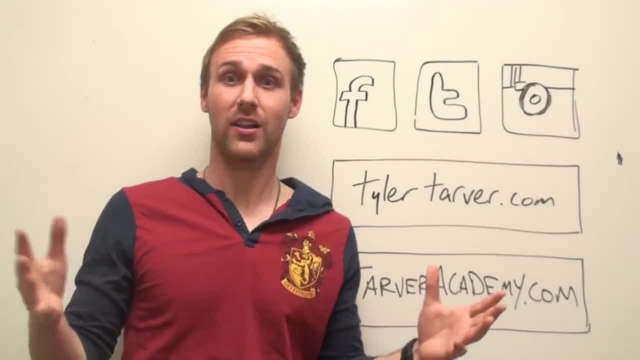 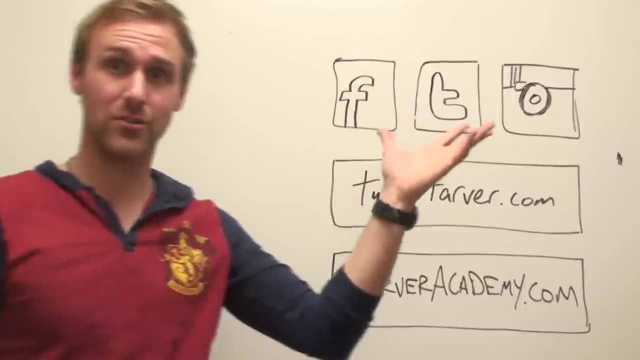 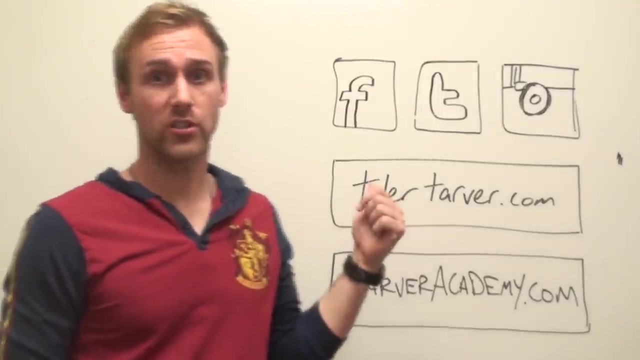 Tarver twittercom. slash Tyler's Harvard, tyler TRT RV, our black gym on Instagram. just search Tyler Tarver once again. but I gotta talk about everything except Facebook. it's Tyler's. okay, did my best, sorry, mom. okay, if you want, you can check out my website, style proper, calm. or if you're on YouTube, you just click this. 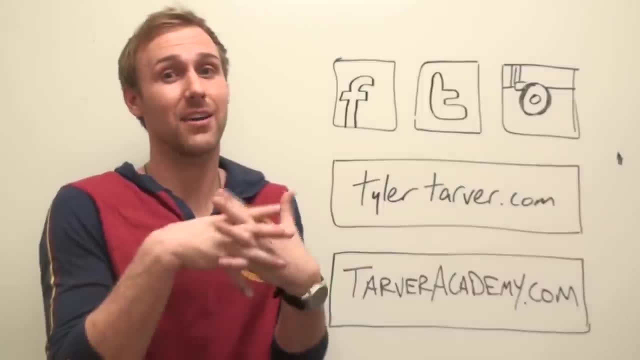 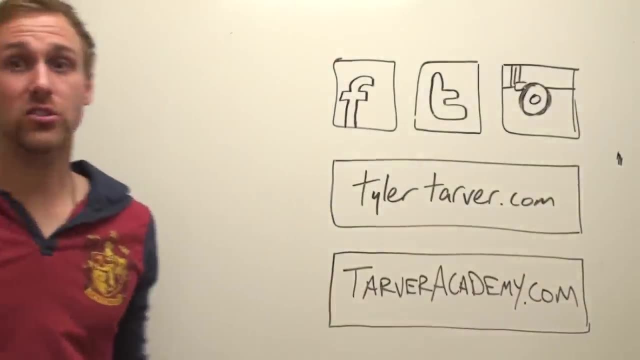 take you to my regular YouTube page where I post videos that are less math and more not math. I try to be funny, I'm just kidding. and then you go to Tarver Academy comm. it's got a lot of math videos. try to organize them for you. 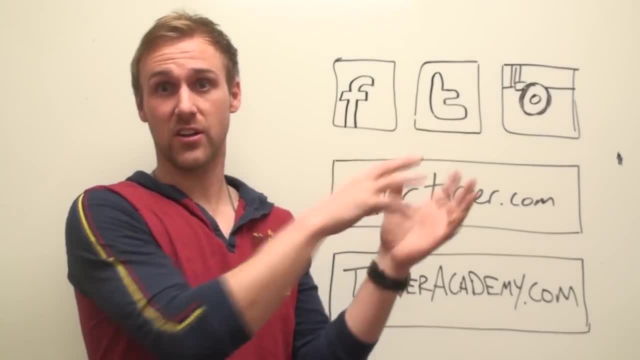 got tons of math videos, little help videos, some that are just off there somewhere- I'm just kidding. and then you go to tarveracademycom. it's got a lot of math videos. try to organize them, for you got tons of math videos, little help videos, some that are just off there somewhere. I'm